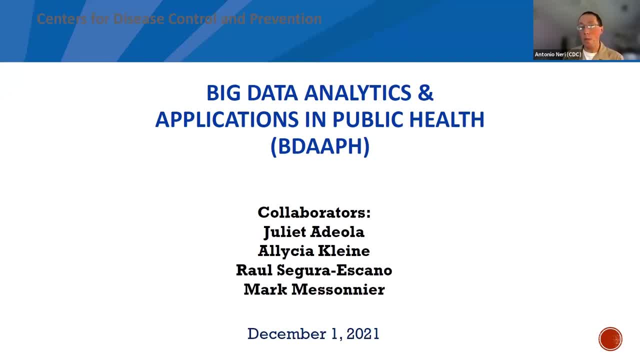 Program or have equivalent public health experience. The Preventive Medicine- Grand Rounds, sorry. the Preventive Medicine Residency and Fellowship is pleased to announce the opening in January 1st 2021. of the Population Health Training in Place Program application for the 2022 class that. 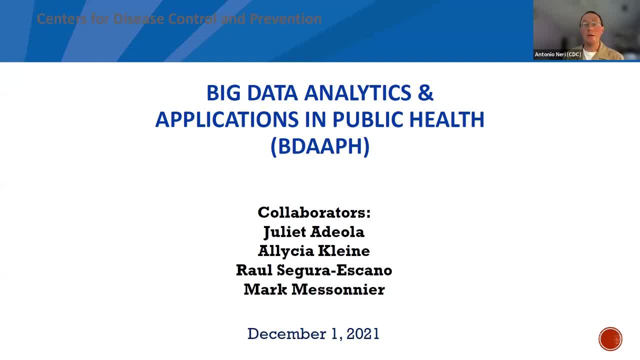 would start in July of 2022.. This year, physicians seeking board certification in general preventive medicine and public health will be eligible to be part considered residents of the CDC Preventive Medicine Residency and Fellowship through the PHTIP program. You can find more. 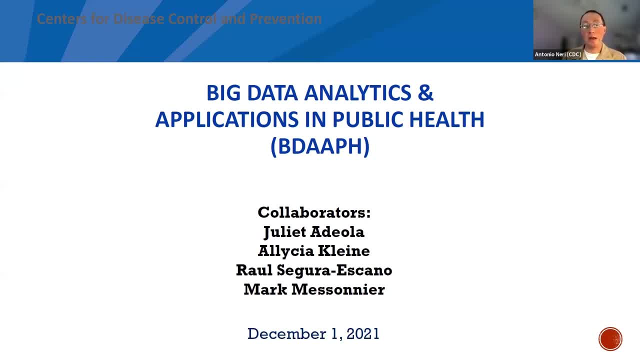 about these two programs on our website, cdcgov. slash prevmedicine. You can see we use Zoom for audio and the presentation and the question box to pose questions. Note that you can pose questions via the text box at the bottom at any point during. 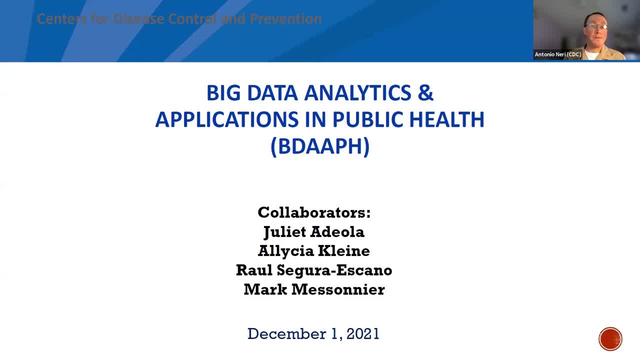 the lecture and those speakers will work on answering them at their discretion. Note: your name may appear associated with the question you pose. If you do not want your name to be associated with the question you pose, then check the box. Submit Anonymously. Continuing. 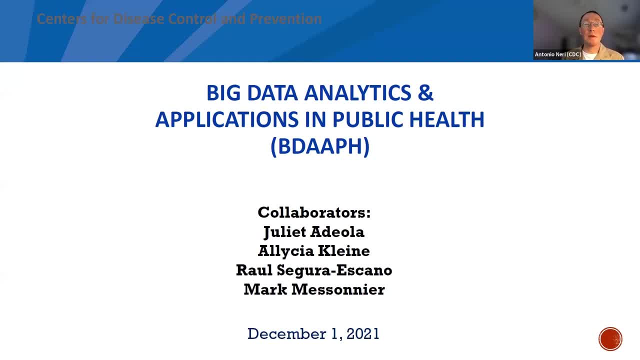 education. credits are available for the live course for up to one month After the presentation date and for the recorded version up to two years from the date of the presentation through the CDC Training and Continuing Education online portal. The course code for this Grand Rounds is all capital letters- CDCPMRF. Again, all capitals, CDCPMRF. 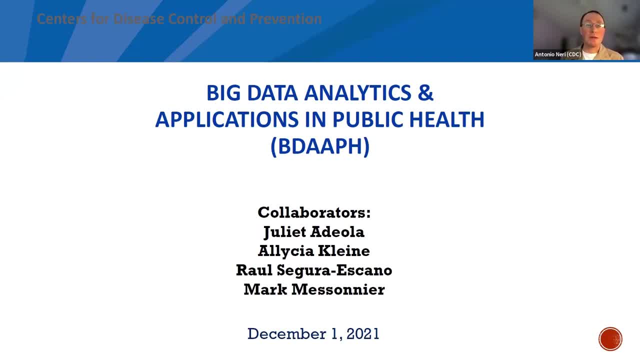 If you have questions, please contact myself or email the program at prevmedcdcgov. Please remember that the views presented by the speakers are theirs alone and do not represent CDC, the Department of Health and Human Services or the US government. Before we start our presentation: 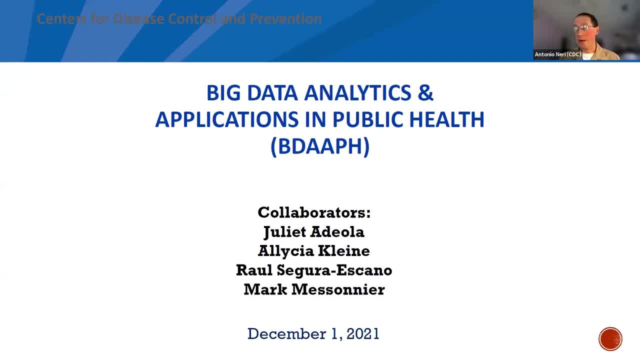 I want to always take our usual moment of silence over this last year and a half or further of the pandemic, just to recognize the friends, colleagues who have suffered morbidity and mortality from COVID and those who have persevered to work so hard to provide care and public health for 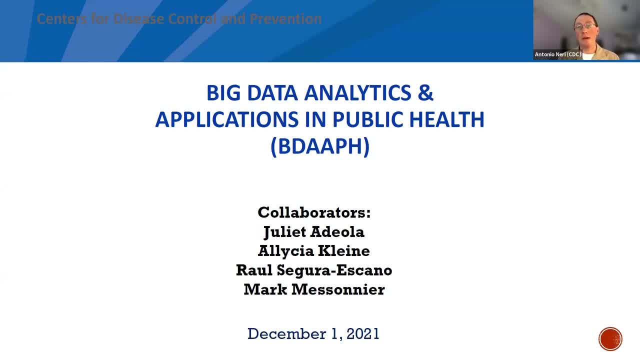 people so they don't get affected by COVID or treat those that have been. Thank you, Okay. So today's Grand Rounds will focus on big data analytics And I'm super excited We have three fellows from different components of the CDC fellowships within our division And I think 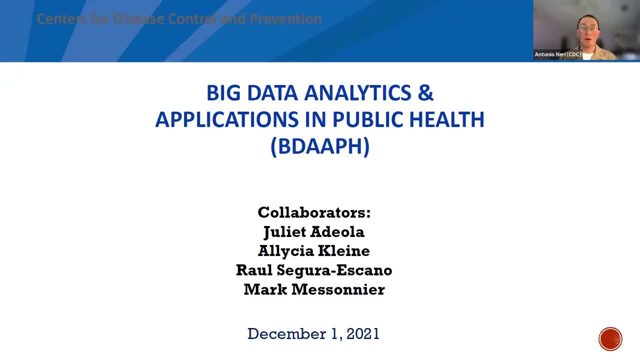 we were talking about it a little bit earlier, but big data is critical. It's increasingly important in this day and age And I can tell you at the agency, I think we have a very difficult time trying to understand what big data, how to analyze it, how to manage it and how to analyze it Not what it is, but what it is, And I think it's a very important part of the agency And I think it's a very important part of the agency And I think it's a very important part of the agency. 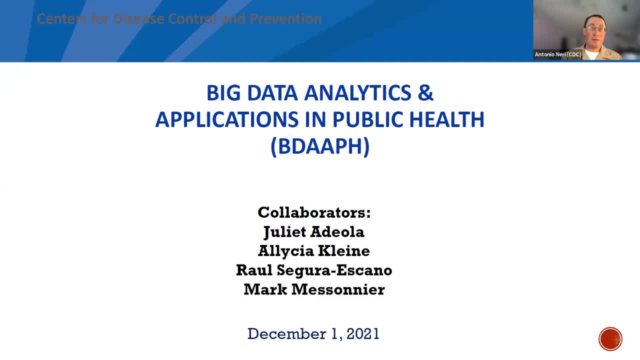 But how to analyze it and manage it, And my assumption is, if we are struggling at CDC to do this, I can guarantee you the state and local health departments that we are engaged to support are doing it as well. So I'm super excited to present our speakers today, and I'll let them 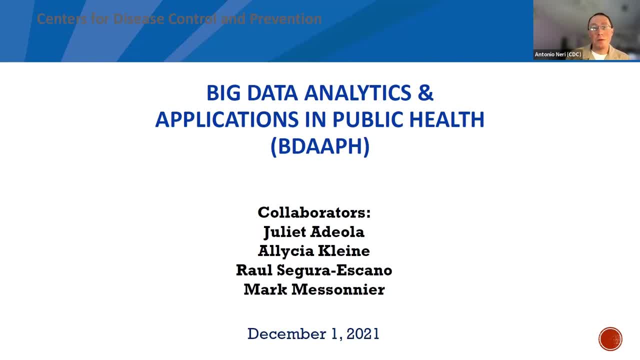 take it from here. Thank you so much for all for coming. The floor is yours. Hello everyone, Thank you for joining us. We are delighted to be here presenting at the Grand Rounds. My name is Juliet Adiola, Myself and my colleagues Raul. 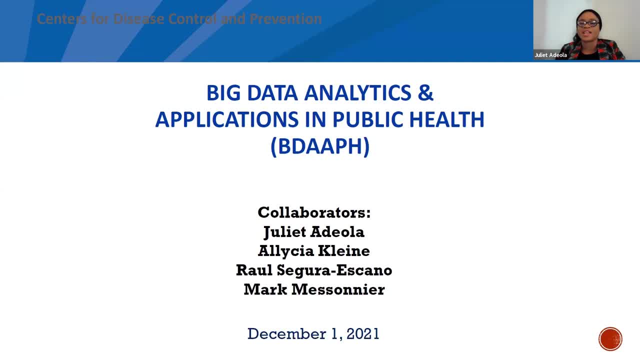 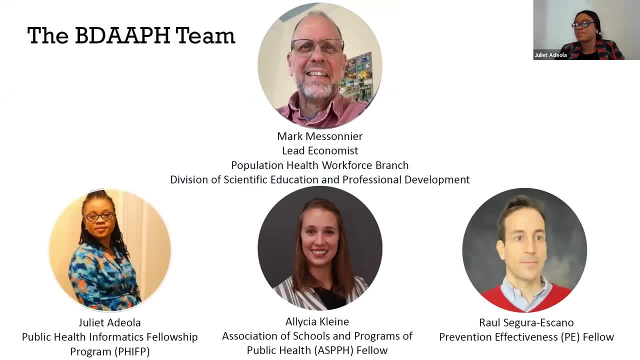 and Alicia will be presenting the big data, analytics and applications in public health. The three of us are fellows belonging to the three different fellowship programs, but we are all located in the population health workforce branch in the Division of Scientific Education and Professional Development within the Center for Surveillance, Epidemiology and Laboratory. 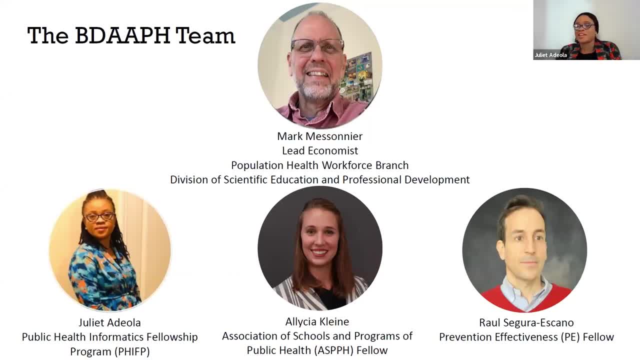 Services. Headshots of the BDAAPH team: Mark Messonnier, Lead Economist Population Health Workforce Branch. Division of Scientific Education and Professional Development. Juliet Adiola, Public Health Informatics Fellowship Program. Open Brace- PHIFP- Close Brace. Alicia Kleiner. 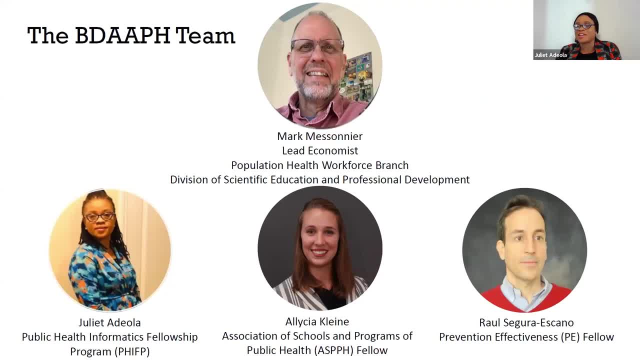 Association of Schools and Programs of Public Health- Open Brace- ASPPH- Close Brace. Fellow Raul Segura Escano- Prevention Effectiveness. Open Brace- PHIFP- Close Brace. To share a little bit about our team. we are under the supervision of Dr Mark Messonnier. 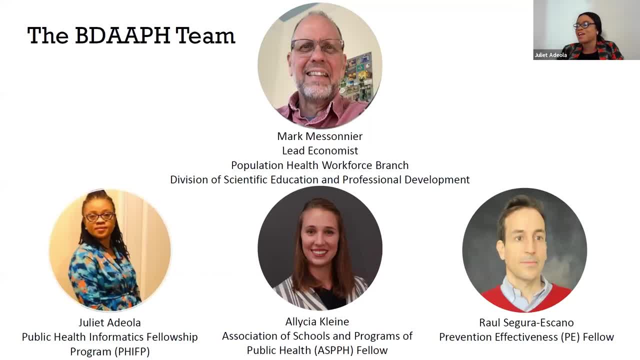 Lead Economist in the Population Health Workforce Branch within the Division of Scientific Education and Professional Development in C-Cells. At the beginning of this year, Mark noted our overlapping interests and brought us together to form a cross-fellowship collaboration within the branch. I'll let the others introduce themselves, but again, 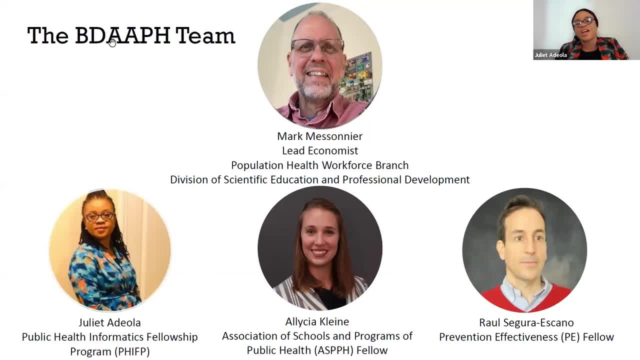 my name is Juliet Adiola. I am a second-year fellow at the Public Health Informatics Fellowship Program. Over to you, Alicia. Thank you, Juliet. Hi, my name is Alicia Kleiner. Thank you for having us today. I am a second-year. 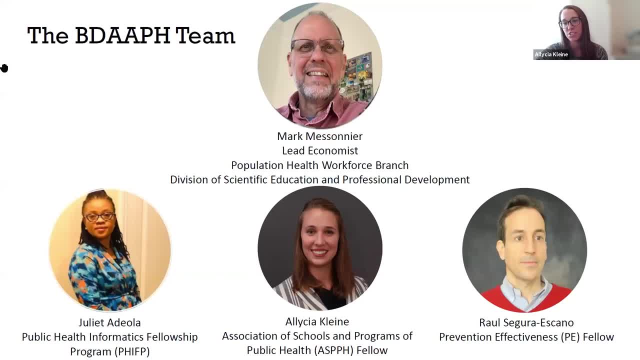 ASPPH fellow which falls under the Academic Partnerships to Improve Health Program, Raul. Hi, my name is Raul Segura. Thank you very much for the invitation to the Grand Rounds presentation series. I am a Prevention Effectiveness Fellow and I am also an Economist by training. 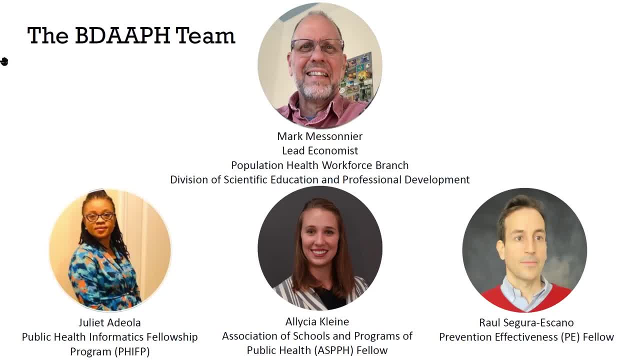 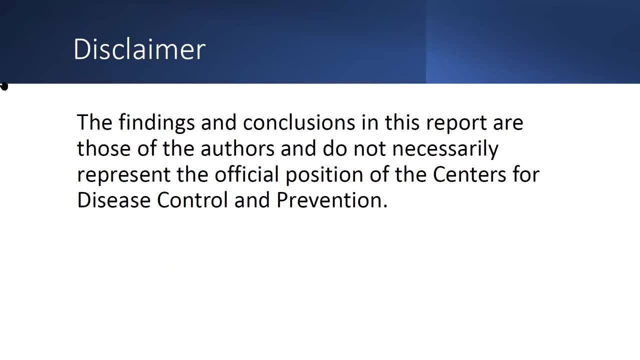 Thank you very much. Thank you for the disclaimer. I would like to also say that we echo that the findings and conclusions in this report are those of the authors and do not necessarily represent the official position of the CDC. Our outline for today during the presentation. 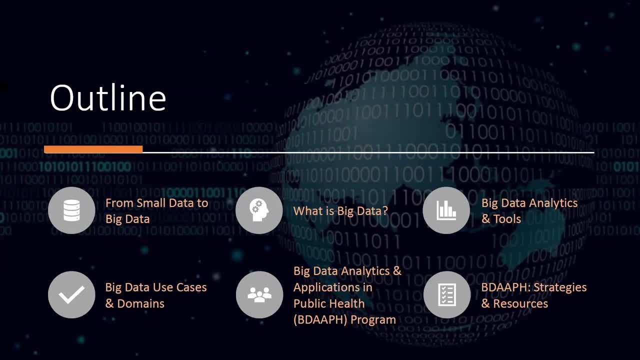 we will be talking about the findings and conclusions of the report and we will also discuss the transition from small data to big data. We would look at what is big data, big data analytics and tools, big data use cases and domains. We will also take some time to talk. 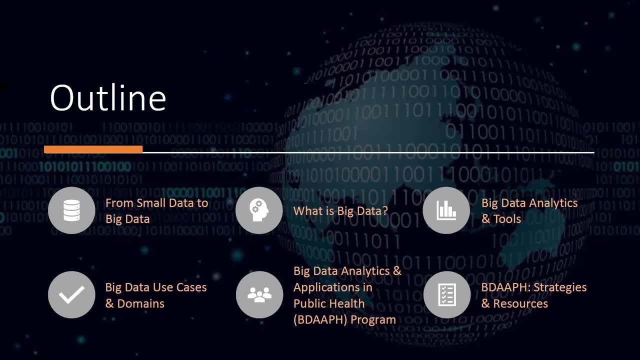 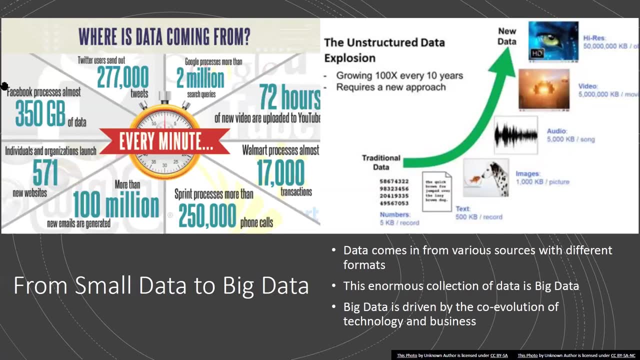 about the big data analytics and applications in public health programs, and also we'll talk about our BDAF strategies and resources. Next slide: From small data to big data. data comes in from various sources with different formats. This enormous collection of data is a great way to learn more about the public health program. 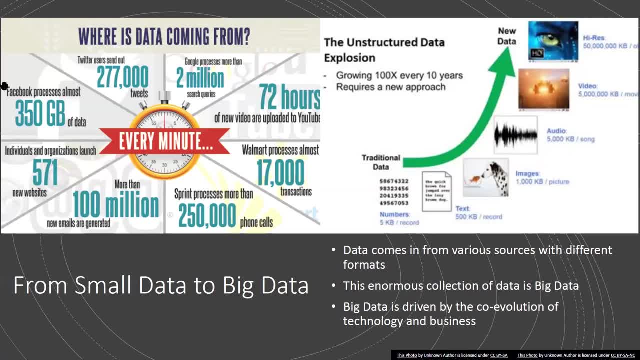 This enormous collection of data is a great way to learn more about the public health program. This enormous collection of data is a great way to learn more about the public health program. Big data is driven by the co-evolution of technology and business. An infographic: Where is data coming from? Every minute, Twitter users send out 277,000 tweets. 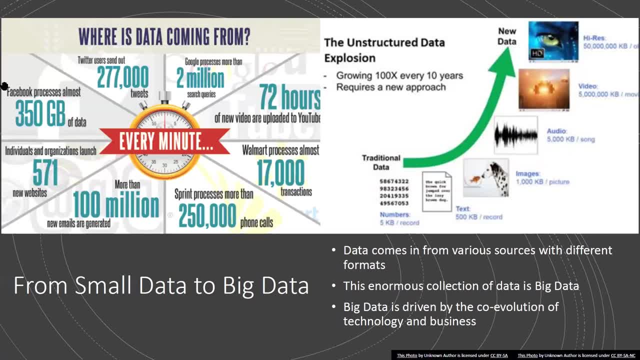 Google processes more than 2 million search queries. 72 hours of new video are uploaded to YouTube. Walmart processes almost 17,000 transactions. Sprint processes more than 250,000 phone calls. More than 100 million new emails are generated. 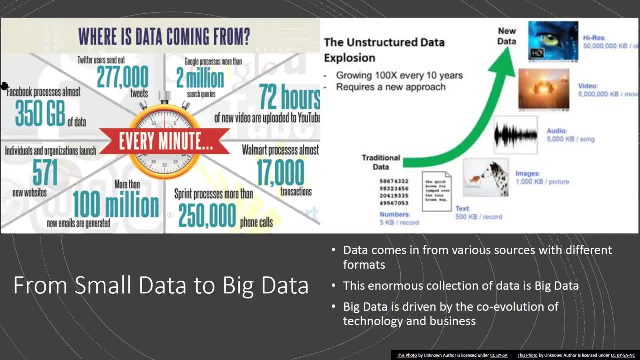 More than 100 million new emails are generated. More than 100 million new emails are generated. generated Individuals and organizations launch 571 new websites. Facebook processes almost 350 gigabytes of data. A second infographic: The unstructured data explosion, Growing 100 times. 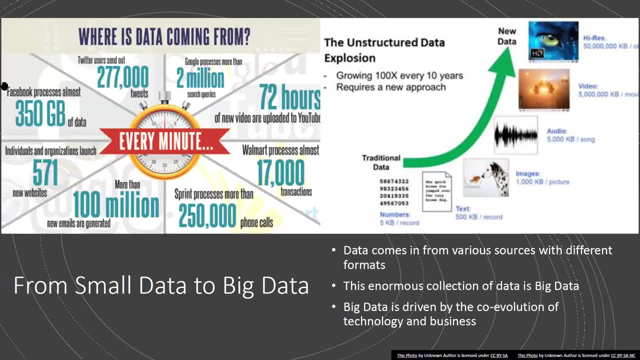 every 10 years, Requires a new approach, An upward sloping area from traditional data to new data. This data includes numbers: 5 kilobytes per record Text- 500 kilobytes per record Images: 1,000 kilobytes per picture. Audio: 5,000 kilobytes per song. Video: 5.000,000 kilobytes. 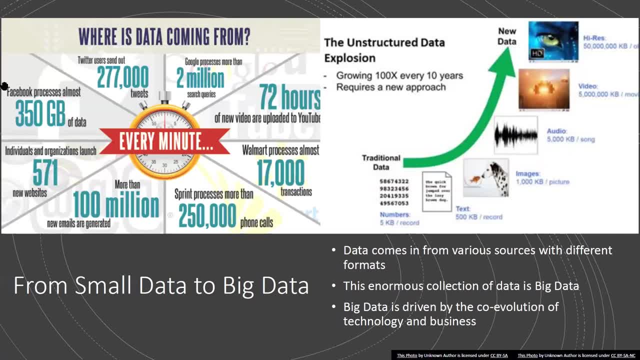 per movie Higher ends 50 million kilobytes. So let's start by looking at where data is coming from. Big data comes from a variety of sources: Machines, people and organizations. Machine generated data refer to data that is being used to generate data, And machine generated data refer 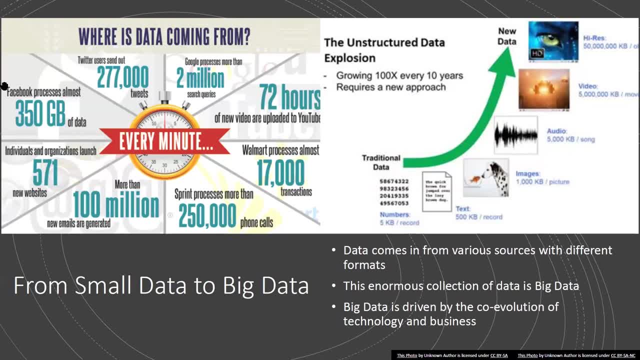 to data that is being used to generate data. And machine generated data refer to data that is generated real time Using sensors in industries, machineries, airplanes or vehicles. Today, there are activity logs that track user behavior, online, environmental sensors or personal health. 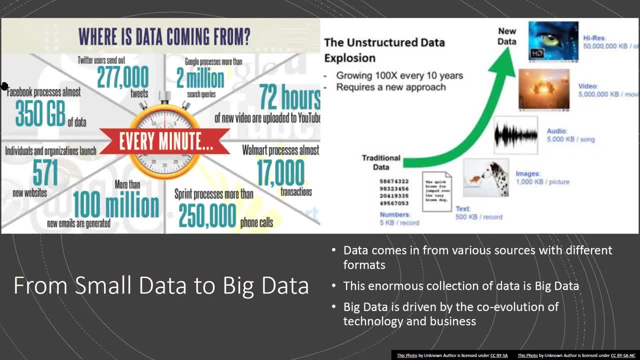 trackers. We can imagine a world of smart devices at home, in our cars, in the offices, city, remote, rural areas, in the sky, even in the ocean. All of these devices are connected together and generating data. Big data also can come from human sources. 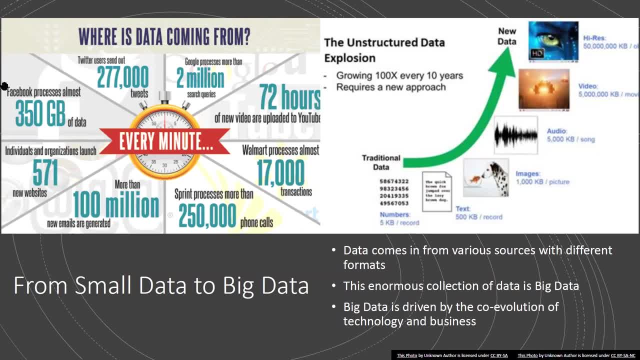 Human sources such as Facebook. as you can see, a lot of people are making different posts on Facebook. Also, you see a lot of videos uploaded to Instagram: photos on Instagram videos, on YouTube. An enormous amount of information gets generated by people. So if you look at the 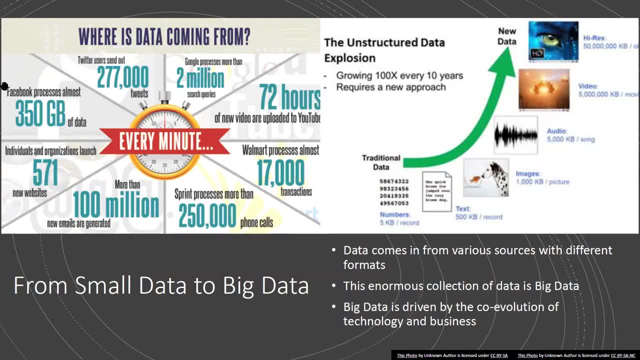 charts, you can see that there are thousands of people, even through blogging and commenting, internet searches, text messages, email and through personal documents. This is what the story looks like today. Before now, traditional data was just mainly data from numbers, text, and then we had images, audio, and today we have high resolution data that actually go in large volumes. We'll talk a little bit about that. Finally, data also comes from organizations. Organizations generate data, which include transactional data, big data, analytics techniques. to address public health problems. I'd like to take a moment to quickly acknowledge those who have been essential to the progress thus far of the VDAC program. The support and guidance that we have received from these individuals and groups has been greatly appreciated. So again, thank you for your time and for your attention. Please don't hesitate to reach out if you have any direct questions or comments, but now we'll open it up for questions. Thank you all for doing that. I very much appreciate it. There is one question in the question and answer box and I have a couple of my own. but I'll let you Answer that one. That seems pretty straightforward. Can you all see that? Yes, The first question: will these slides be available somewhere? Oh, we'll answer those top two ones. but who? the target audience was for the survey and the curriculum. Okay, Thank you very much, Thank you, Thank you. So our target audience are fellows, CDC fellows, excluding the ORISE fellows, for now, for our introductory course. And then there's another question that came in that asks sort of about future fellowships. with public health professionals looking to gain experience in big data analytics- And I actually pose that in a bigger question. Can you talk a little bit about Other opportunities to train in this area? How can you get more training in this area? Okay, I'll turn that over to Raul to respond and then I can chime in. Yeah, So basically we have identified several fellowships that could be potential receiver of data. receiver of it, i mean, might be interested in this type of training, but we are open to any other. students or potential fellows that would like to join, also not only fellows, but anybody interested in this topic, which i we believe that is very important and very relevant in today's world. so we basically, like i said, we are open to to any kind of audience that is interested in in this. in this training. i'd like to also add there that, um, thank you, ralph, for that. so, um, we hope that our courses would be available on um public spaces, especially within the cdc platforms, that people can easily go and take those courses and, as much as possible, as we kick start, we would also expand our reach. thank you. i think- and correct me if i'm wrong- most of the opportunities we're talking about are internal to cdc at this moment, right? is that correct, raul and juliette? yes, yes, at this moment. but we also have um, a plan, uh, a long-term plan to make our courses available for global audience. on, coursera or really, or on any other learning platform that people can actually reach. and and then maybe i'll take that one question a little bit further: if you, as you develop this understanding of big data analytics and the workforce capacity, can you talk a little bit about how non-cdc entities, particularly public, and private and academic partners, and particularly state and local health departments, can prepare their workforce in to to both collect and analyze big data analytics. how do you want to start? but i can also um start. i think one preparation that i would say for now is to also increase. capacity, which we are trying to bridge capacity gap, knowledge gap, using these trainings. also increase um training on big data ethics also. it's one other place that i see that organizations can start to prepare themselves. you know talking about data going to shape, governance and access. those are very important um aspects that people need to. prepare themselves also with all of this data that we have access to raul or alicia. what do you think? yes, i mean a data access- is a critical part of the big data analytics and we we acknowledge that part, and so we have a cdc, we have the cdc data hub that contains and provides a very very important data. i mean the quality data that we we envision for for this type of project. but i think that what juliette has mentioned before, that ethics is an integral part of the big data analytics and so important aspect of the usage of data, And this is something that has been in the community. I mean being everywhere else- is talking about the limitations of between having the thing that you need so much data, so much volume of data before you can call it big data. But from the discussions today we can see that that is not always the same the truth. You're looking at the five Vs of big data. Now we know that it's not only how large, but how complex and you know how fast and quality of data and then, of course, value added. So we have better understanding. you know, and then sometimes also people misconstrue And think that big data talk is relational databases, which is like traditional data into a document that I think I mentioned during my presentation that would be accessible upon request. So in that particular slide we mentioned seven applications of artificial intelligence for COVID-19.. And one of them, for example, would be in terms of for. example, drug and vaccine development can be used. artificial intelligence can be used to for drug and vaccine development in speeding up the testing process. This is something that is probably now in the media, has been recently in the media as a new new COVID-19 new. how do you? say this, This Delta variant And the Omicron variants appear. So this is something that I think artificial intelligence can really have a big impact on this particular aspect of vaccine development And in that particular slide that we compiled the information from articles, we selected seven of them. but probably there are more we might not be aware of, But this is just to show that there are a large number of applications of artificial intelligence, the tools on machine learning, on COVID-19.. Julia, did you want to add to that? or Alicia? So you feel good about that too, that's fine. The other question is about two questions that sort of stem off of one that someone submitted. One is representative activity, So big data and how, what it represents. I wonder if you could talk a little bit about that. For the last 18 months or so I've been helping out with the telehealth operations at the agency. One of the things we've run into in big data sets is how representative the data is, And I think particularly in what are termed now population health companies. the abstract data from individual siloed electronic health records and aggregated also de-identify it. It's been very difficult to look at how representative they are of different populations And I was wondering if you could talk a little bit about that and have a follow-on question to that. What's one of those